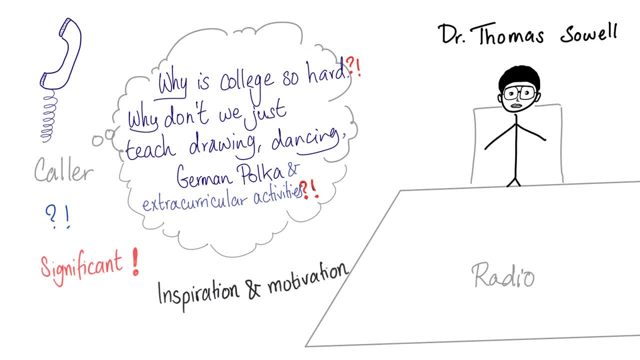 there was Dr Thomas Sowell and he was receiving a call, And the caller asked a very sophisticated question: Why is college so hard? Why don't we just teach Drawing, dancing, German poker and extracurricular activities? To which Dr Sowell replied in his 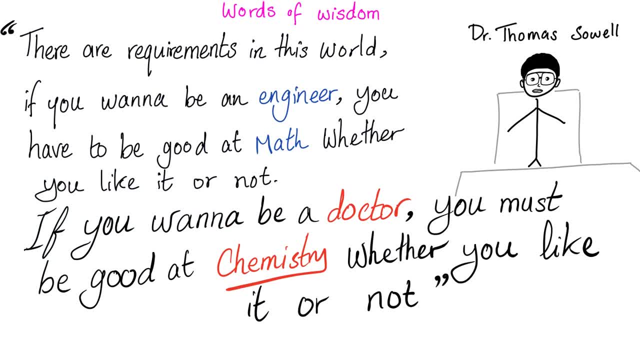 infinite wisdom. there are requirements in this world. If you want to be an engineer, you have to be good at math, whether you like it or not. If you want to be a good doctor, you must be good at chemistry, whether you like it or not. I know this sounds brutal. I know it has just shattered your 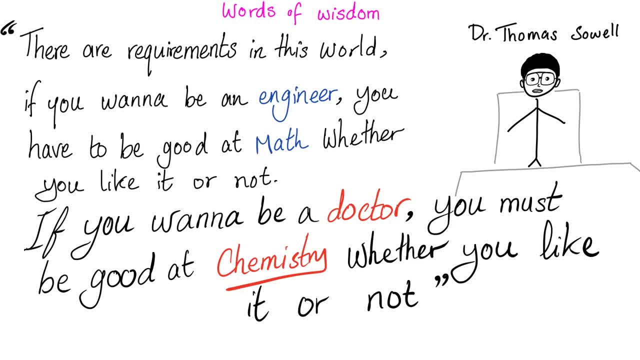 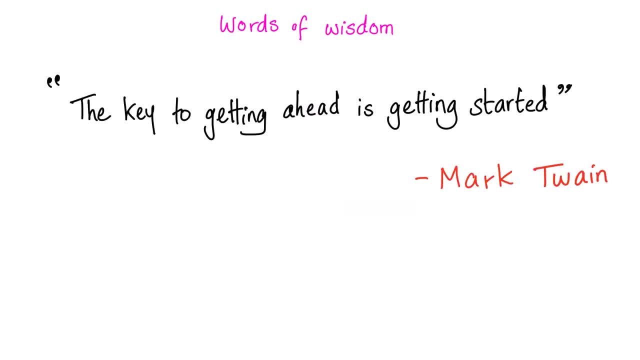 world. but it's actually true. I'm not here to massage your back with warm oil while you kill the patient. It's not going to happen. But before you get mad at me, here's the good news. The key to getting ahead is getting. 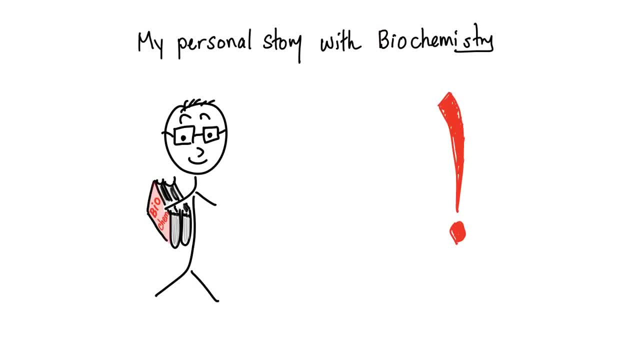 started, You can do it. So here's my personal story with biochemistry. In my first year of medical school, I hated biochemistry the most, more than any other subject. Yet my score on biochemistry was the highest compared to any other subject. So the harder I worked, the more I 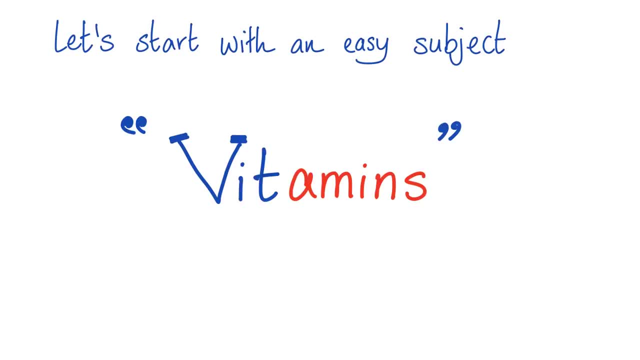 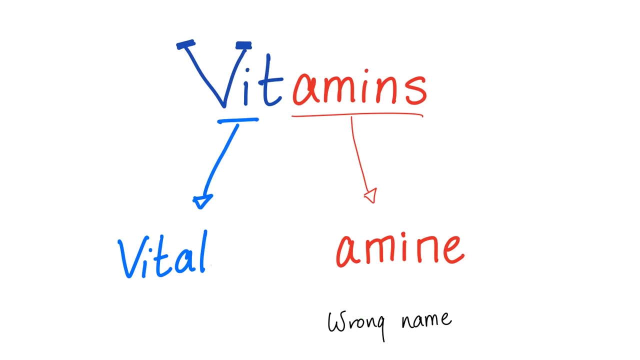 got, And you can do it too, Instead of just starting with enzyme kinetics and make you like hate yourself. let's start with a very easy topic called vitamins. But first, where did this word come from? Vitamins? What So the word vitamins came from two words: vital and amine, which is 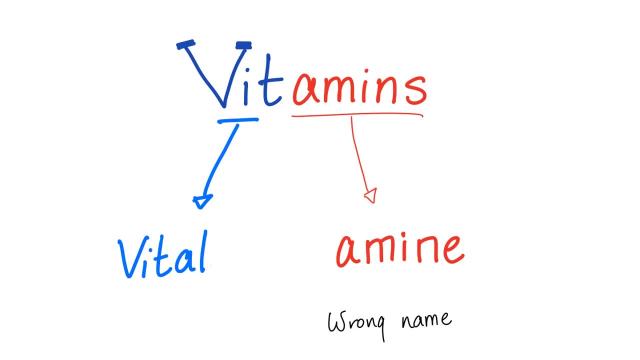 actually a wrong name, because vitamins are not actually made of amines. Oh, so why do we call this? It's a wrong name. Like in the past, we thought it was a wrong name, So let's start with amine. We thought that they were amine, Actually the only vitamin that could be considered as. 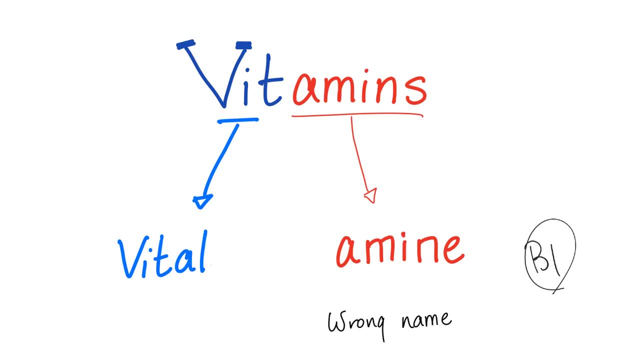 amine is vitamin B1.. Other than that, I don't think that they are amine, But the name just remains And in the past they used to write it like this: A-M-I-N-E-S. So if your professor 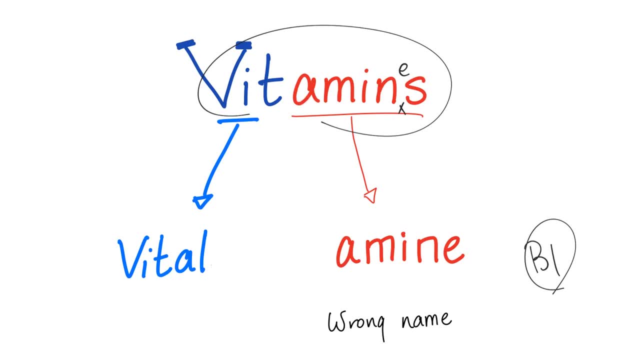 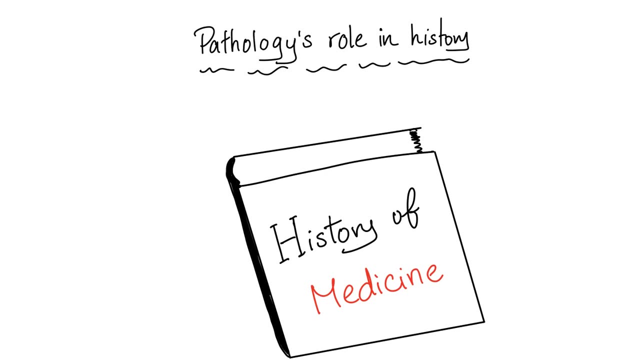 still uses vitamins and writes I-N-E-S. it means that he has been alive since Magna Carta. Now let's talk about the role of pathology in the history of the world, because nobody talks about pathology in the history of the world, So let's start with the role of pathology in the 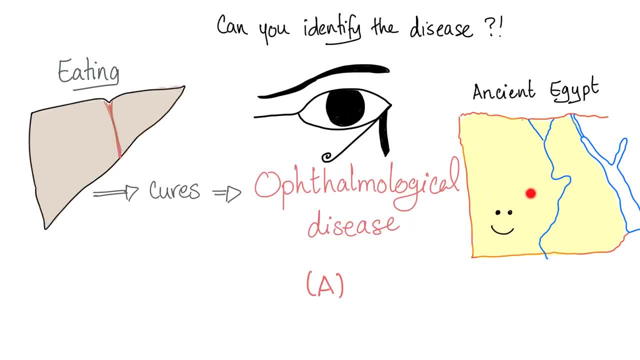 history anymore, But it's actually fascinating. Since I'm an Egyptian guy, let's start with ancient Egypt. They realized that eating liver can actually cure, slash, prevent an ophthalmological disease. Now I'm not going to tell you which ophthalmological disease it is, because now it's. 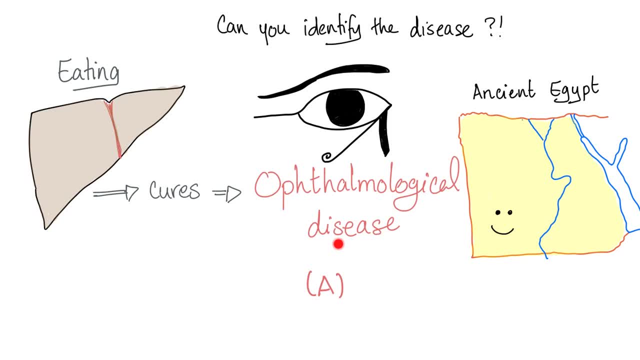 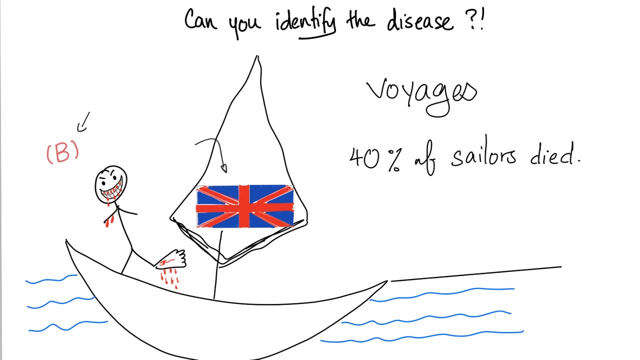 going to be so easy. The question is, what is the ophthalmological disease that could be cured, slash, prevented, by eating liver or liver oil or something like that? Now let's talk about another disease. Let's go back in history to the time of Great Britain, just. 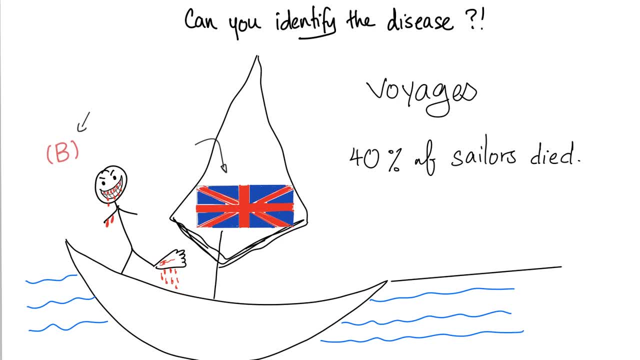 after the Renaissance and around the era of the Industrial Revolution. Britain prospered for many reasons: For its geographical location, which was far away from Europe. Therefore they were less involved in wars. They were the first people to throw away the monarchy. They developed capitalism. 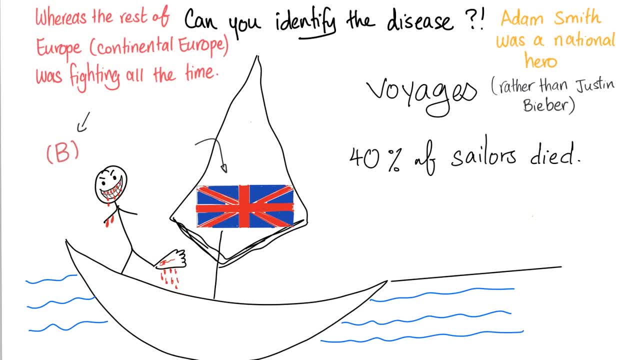 which is free market economics. They developed separation of powers. So at that time you have the executive branch, which is separate from the legislative branch, which is separate from the judiciary branch, And those judges actually referred to the law. They did not. 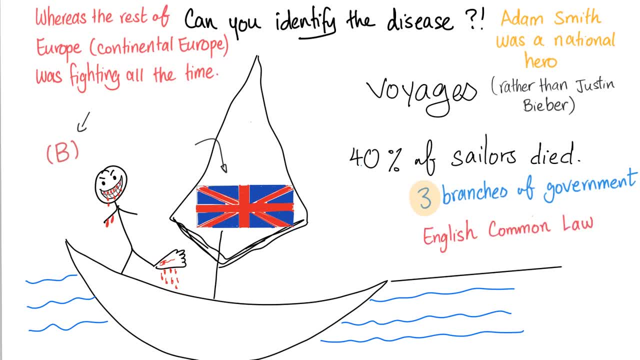 just legislate from their opinion or from their wishes. They actually followed a written law plus legal precedent which provided a great framework for people to just work in Britain. Then they prospered, And after they prospered, they just went everywhere Through these famous voyages, some of which were political, such as British colonialism, Others were 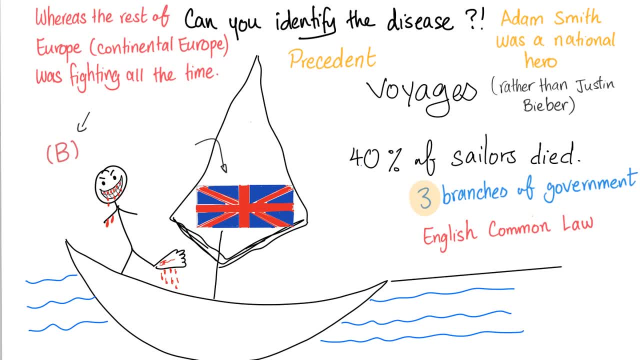 scientific, such as the famous voyage where Robert Fitzroy took Charles Darwin with him to the Galavagos Island. I think Now let's forget about this. They realized that the most severe risk to their sailors was not the enemy: It was a disease that caused the sailors to bleed from their gums. 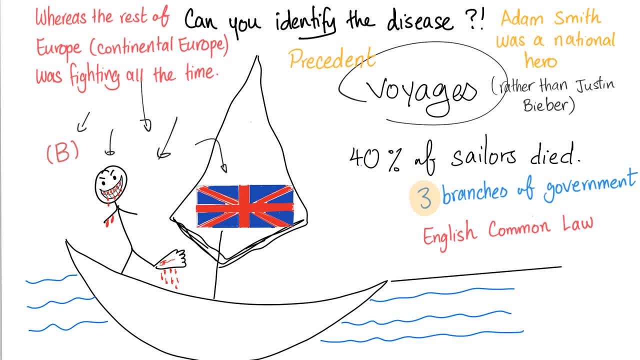 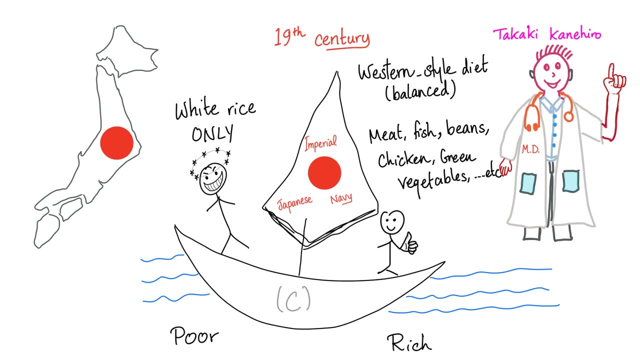 bleed From their skin, have wounds that do not heal And it was crazy- About 40 percent, or even half, or sometimes two-thirds of the entire ship died from this disease. What is the disease? Let's talk about a third disease In 19th century Japan, in the Imperial Japanese Navy, Dr Takaki Kanahiro. 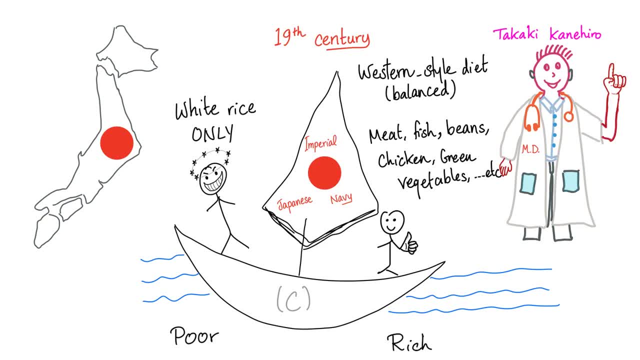 he was trained in Britain, And this is relevant because at that era, only Europe was actually advanced in medicine. Like I'm Egyptian, Do you think that in the 19th century we had any doctors who actually contributed to humanity regarding medicine? No, We only had barbers. The first. 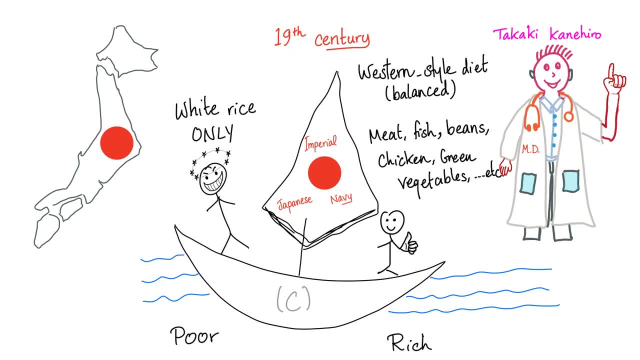 medical school in Egypt was actually in the 20th century. In the 19th century they were just barbers. They will cut your hair and perform phlebotomy and remove your black vials in just one visit. That was about it. Anyways, back to Dr Takaki Kanahiro. He realized that you know. 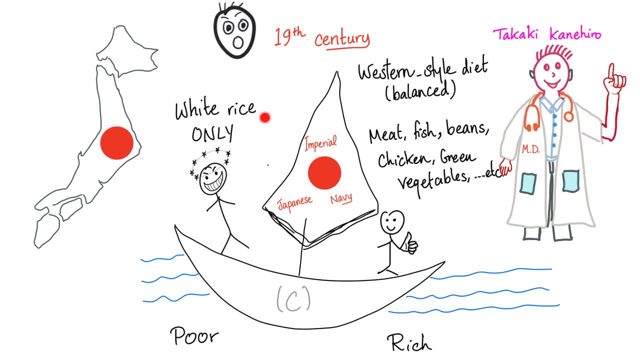 on the Imperial Japanese Navy. there were two groups of sailors. The first group, they were poor. They could only eat white rice only, And that was it. The rich sailors could afford a Western-style diet which was more balanced: They had meat, fish, beans, chicken, green vegetables. 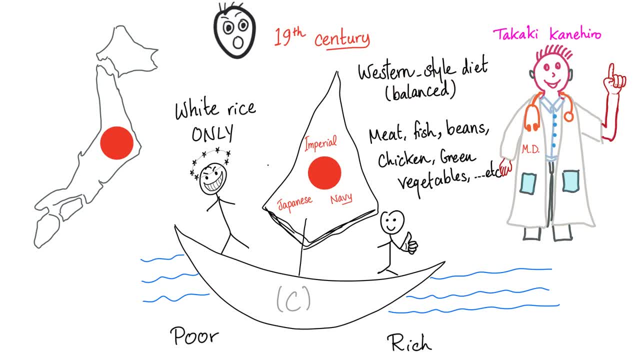 butter, etc. etc. Oh, is that what you mean by Western-style diet? Yes, we're talking about the 19th century. We're not talking about your venti soy macchiato with mocha drizzle. okay, Just get your head out of your sphincter. The poor sailors developed a wide variety of weird. 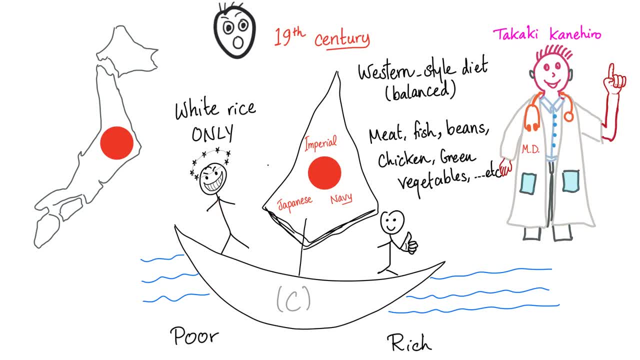 symptoms. Some of them were confused. Some of them could not walk. They had ataxia. Some of them had visual problems or ophthalmoplasia. Others had memory loss. Others had personality changes. Others developed muscle wasting. Some of them developed a high-output cardiac failure and even 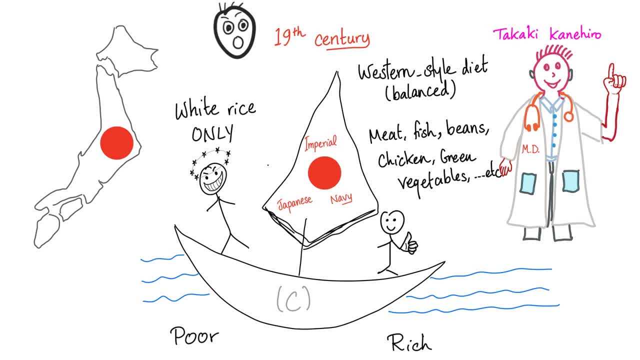 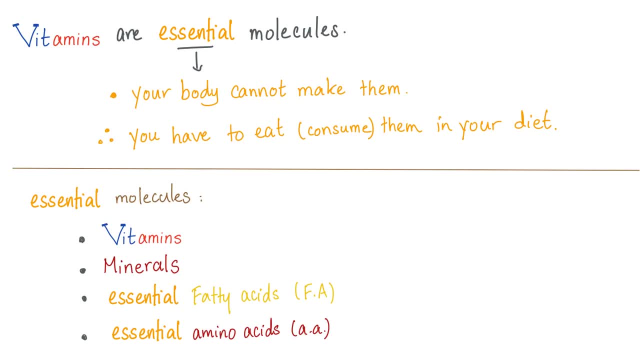 pitting edema. What is this disease? Please let me know in the comment section. Vitamins are essential molecules. What do you mean by essential? I mean your body cannot synthesize them. Therefore, you have to eat them in your diet. And, by the way, 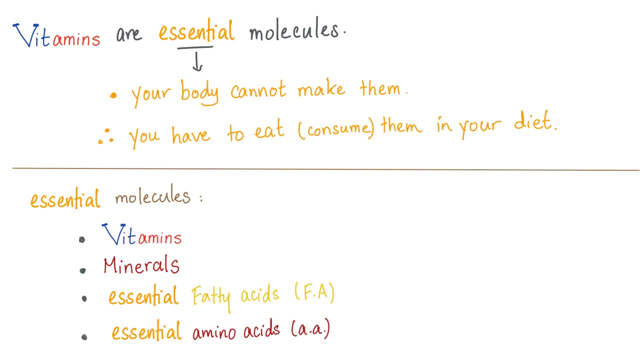 these are the essential molecules that you have to consume in your diet: Vitamins, minerals, essential fatty acids and essential amino acids. When we say essential in biochemistry, we mean: A- your body cannot synthesize it, and B- you have to eat it in the diet. Do not confuse this with 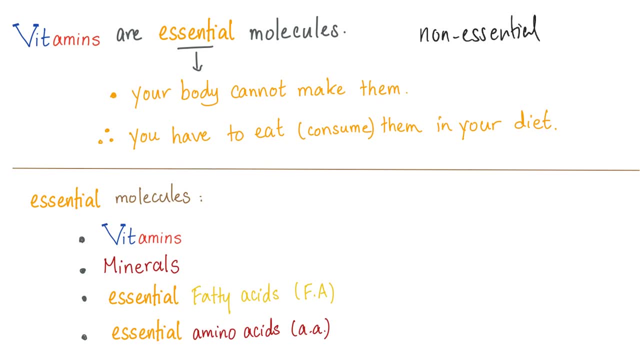 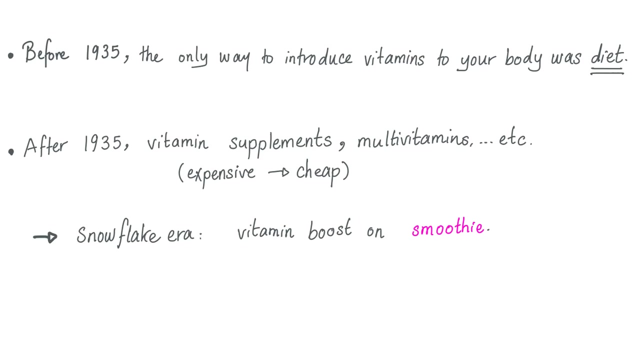 non-essential stuff. Non-essential means your body can synthesize it. You do not have to eat it in your diet. And then there's something weird in between called semi-essential, which is another topic for another day. A history lesson Before 1935, the only way to introduce vitamins into. 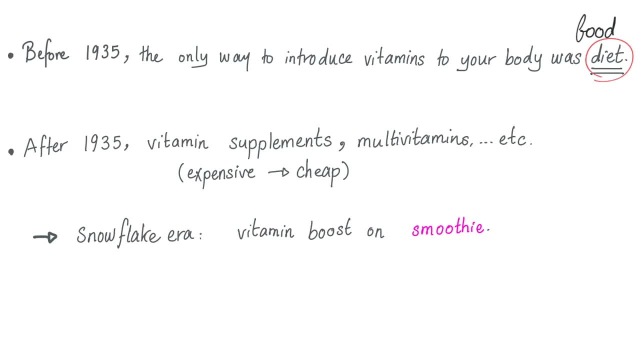 your body was through the diet period. That was it. But after 1935, vitamin supplements were invented And now we have multivitamins and vitamin B complex in a bottle, etc. etc, etc. And today we live in the snowflake era. You can actually add some vitamin boost to your smoothie. So when you 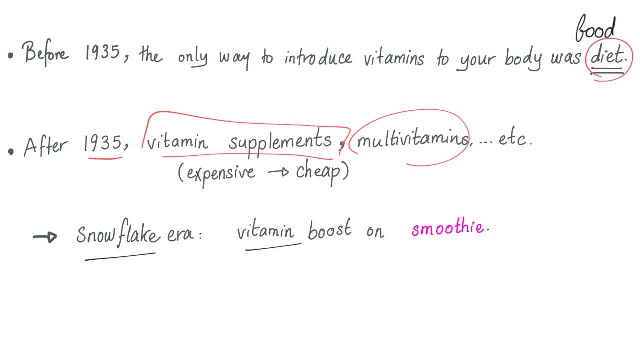 say: oh, I'm a natural person, I eat a natural diet, All natural, No artificial ingredient. And, by the way, I add some vitamin boost to my smoothie. You're a hypocrite, Because if you add a boost to your smoothie, it's not natural by definition. And you are not the only hypocrite. 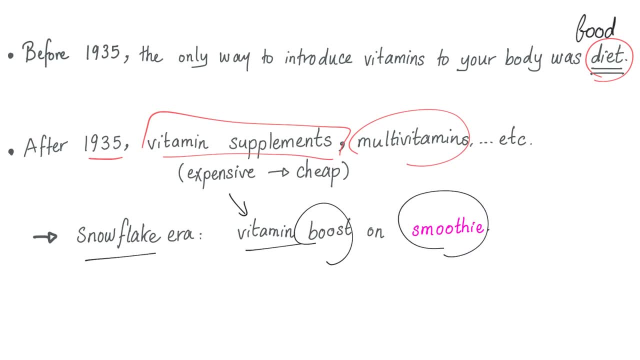 in town. The guy who is selling you the smoothie as quote all natural is lying Because he added a vitamin boost. But the word all natural has become a marketing gimmick Because all of you guys fall for: oh, it's all natural, non-GMO, gluten-free, vegan, lactose-free, whatever, free. 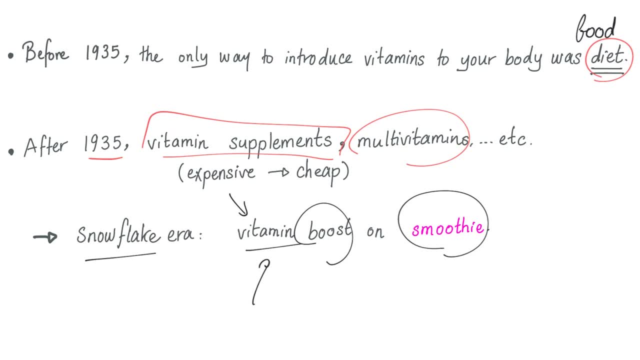 ethically sold like stuff that sounds good but means actually nothing. And as of any other drug, those vitamin supplements started as expensive and then they became cheap. Why? Here's the reason. Are you ready? Supply and demand. Economics 101.. Economics is. 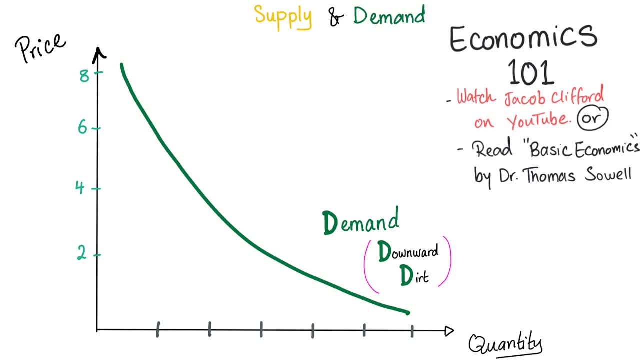 the scientific study of scarce resources which have alternative uses. First let's talk about demand. I have mnemonics in economics too. Demand is downward sloping and it's going towards the dirt, to the ground. D with a- D, There is an inverse relationship between demand and demand. 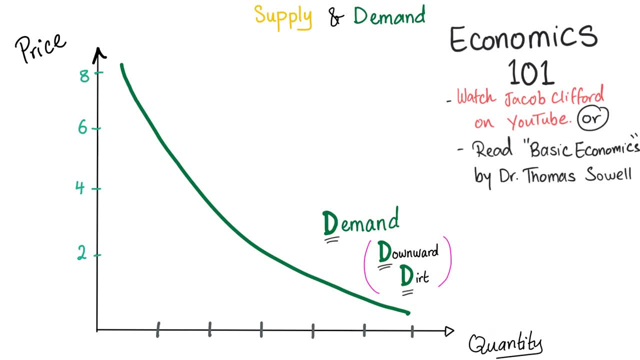 Between the price on the y-axis and the quantity demanded on the x-axis. Translation: let's say that the price of the iPhone decreased from $800 to $100. What's going to happen to the quantity demanded? Follow the curve, baby. People will demand more iPhones because now they are more. 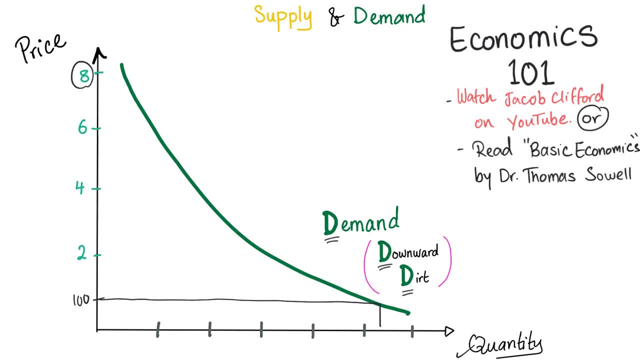 affordable. The opposite is also true. If the price of the iPhone increased from $800 to $8,000, what's going to happen to the quantity? Demand is going to decrease. People will not buy as much iPhones and they will buy many. 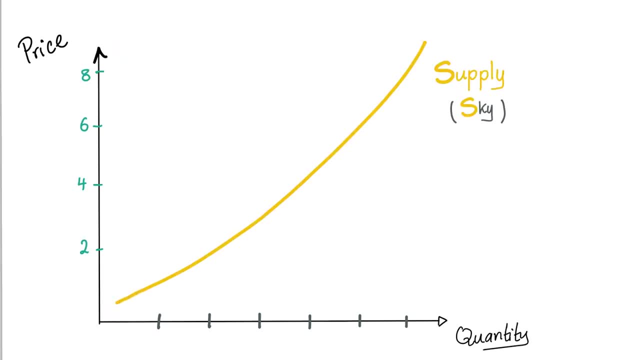 Androids, for instance. Now let's talk about supply. Supply is to the sky. There is a direct relation between the price and the quantity supplied. Let's say that the price of cars increased dramatically for some reason. Now many people will start their own businesses and their 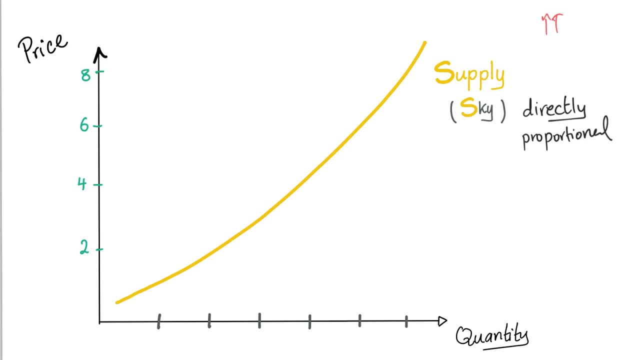 own car companies, because now it's very profitable to make cars. So when the price increased, the quantity supplied has been increased. It's called common sense When the doctors- let's say doctors- are now being paid tons of money, way more than before. 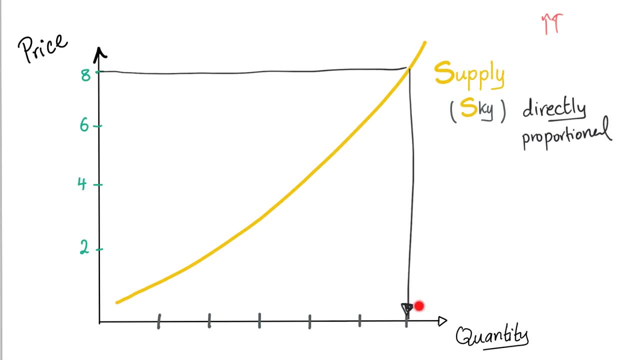 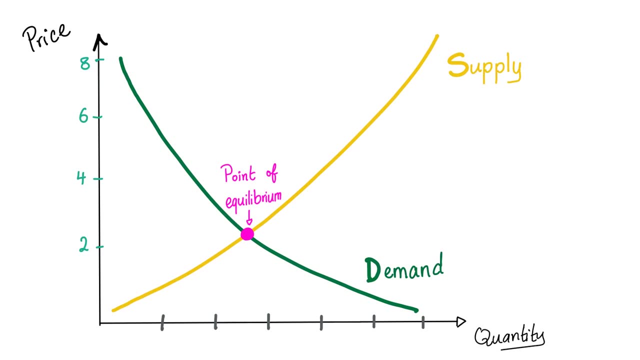 what's going to happen? More people will apply to medical school and you'll have a greater supply of the quantity of doctors. If you leave the market alone- hence free market- it's going to reach this sweet spot called the point of equilibrium. At this point, 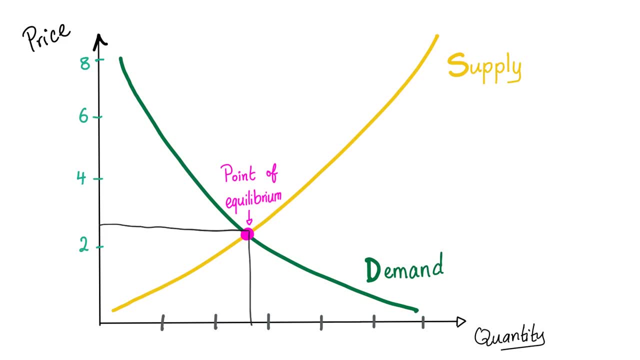 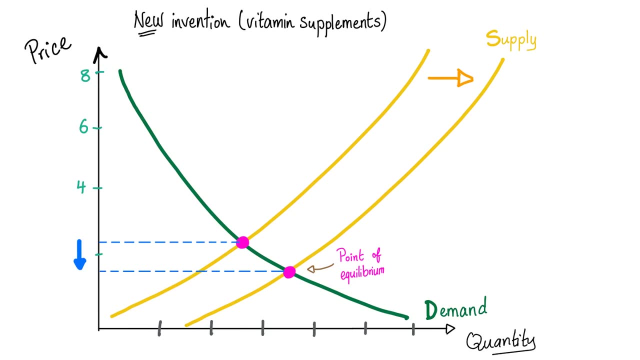 there is a certain price and a certain quantity demanded and or supplied, But then, similar to your oxygen hemoglobin dissociation curve, the supply curve could be shifted to the right when you are increasing supply, If you remember your oxygen dissociation curve shifting to the right. 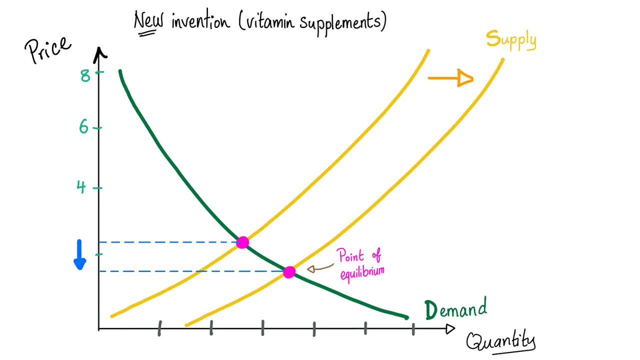 means what? We are increasing the release of oxygen to the tissue. What are the shifters of the oxygen dissociation curve to the right? Increase carbon dioxide pressure, increased hydrogen ion concentration, which means decrease pH, increase temperature, increase altitude and increase 2,3-DPG. Fine, What will shift the supply curve to? 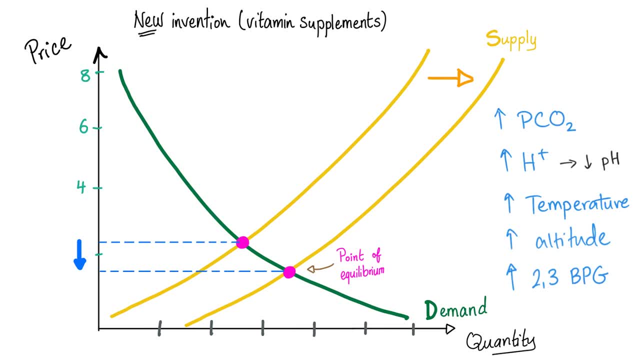 the right Something as new technology or new invention, such as a new discovery, slash invention of vitamin supplements. Now, for the first time, we can actually do vitamin supplements And, as you know, they will start expensive And then every single business. 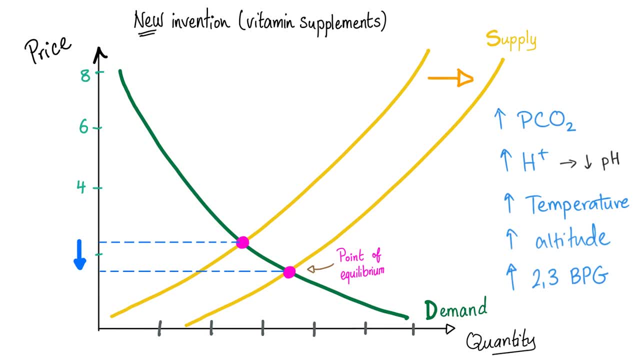 person will start to buy vitamin supplements, And then every single business person will try to start his own drug company, or at least be part of it. What will happen when you shift the curve to the right, because now you have an increased supply of vitamin supplements? 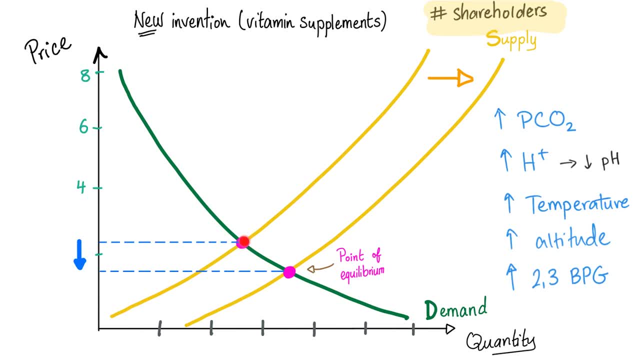 this will lead to a shift of the point of equilibrium from here to here. And if you look at the y-axis, what happened to the price? It decreased from here to here. That's why anything that starts new starts expensive and it gets cheaper most of the time. The first computer was 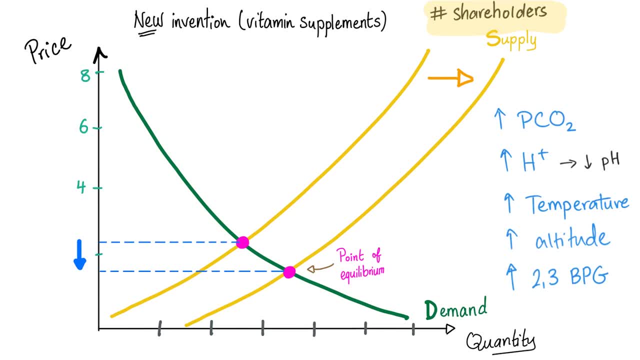 very expensive. Now, if you look at the y-axis, it's very expensive. And if you look at the y-axis, it's very expensive. And if you look at the y-axis, it's very expensive. Now every one of you can have one. The first car was super expensive. Now, on average, every single. 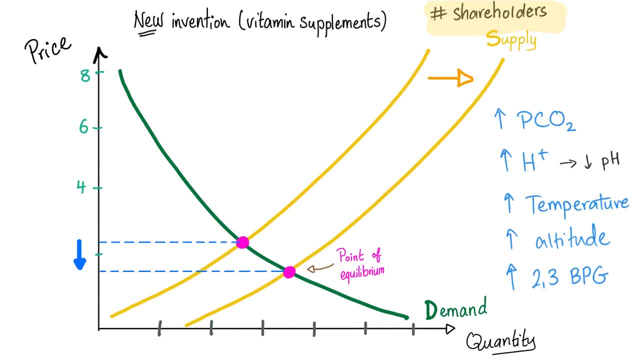 person has a car Today. as of this moment, Ivacaftor, which is a CFTR potentiator, a medication used to treat cystic fibrosis, is super expensive. Give it some time. the patent will expire, the supply will increase, the price will go down, naturally, And the 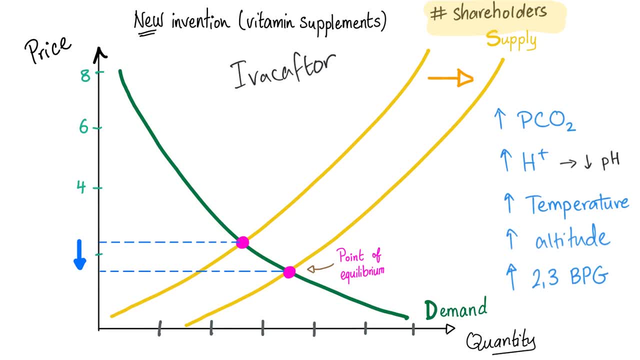 beauty of the law of supply and demand is that it's universal. It's universal, It's like the law of gravity: It works everywhere, whether you like it or not. So when you say, oh, medicosis, you don't know about me, I live in New Zealand, It doesn't apply here, Really. 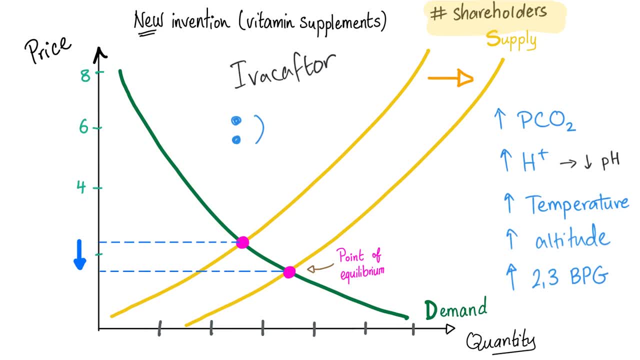 let's not do this. Saying that economics only apply in America is like saying vitamin C is only good for evangelicals. I mean, it's a non-sequitur. Get your head out of your sphincter Now. let's say that all of a sudden, we have a politician with good intentions and he said: 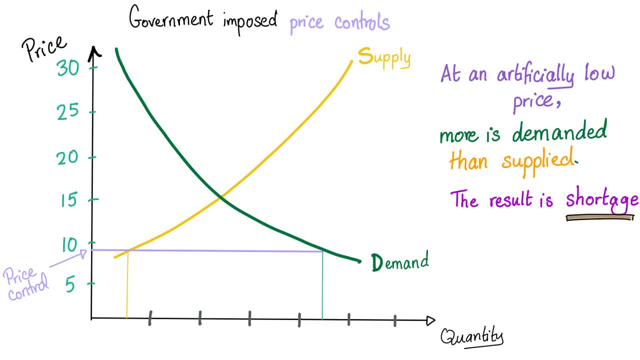 those big pharmaceutical corporations. Those big pharmaceutical corporations are evil. We should impose price controls and control the price so that these companies cannot charge you more than $10 for your medication, because every person deserves a medication. Okay, now look what will happen. Follow the. 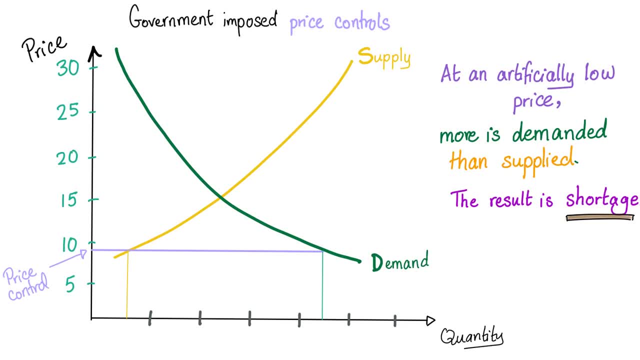 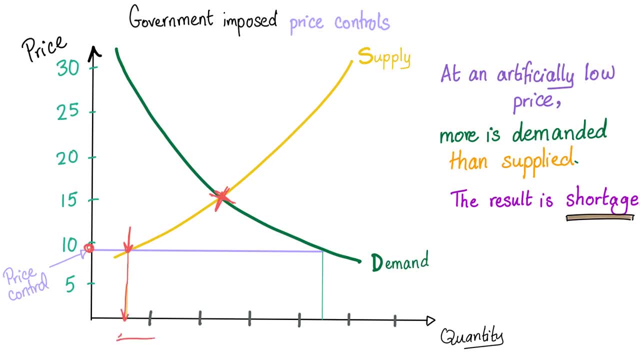 going to go down. Follow the curve. The intersection is here. The supply has decreased And instead of here, as naturally, you have decreased the supply- What's going to happen to the demand when you artificially lower the price? Follow the green curve: It intersects. 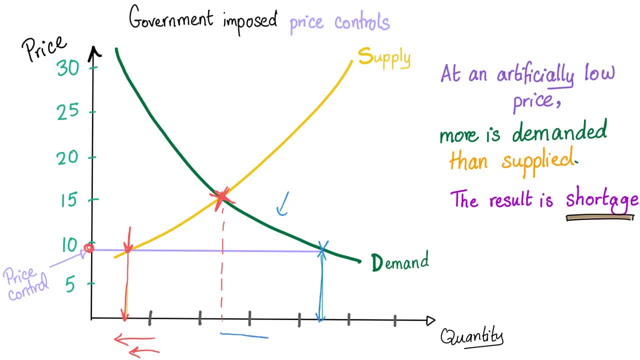 with the purple curve here Go down. The demand has increased from here all the way up to here. When you have a situation with increased quantity demanded but decreased quantity supplied, it's called a shortage. Therefore, here is an economic rule: At an artificially low price, more is demanded than supplied. The result is: 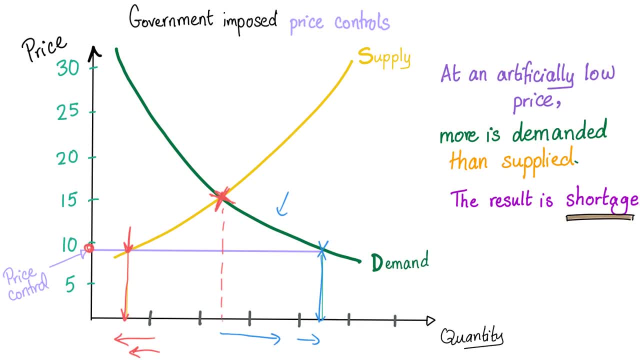 shortage. If this politician did that for insulin prices and fixed them at an artificially lower price, you will have a shortage of insulin. Take it to the bank. You'll have more patients who need insulin and very few companies who are willing to actually make the insulin because it's not. 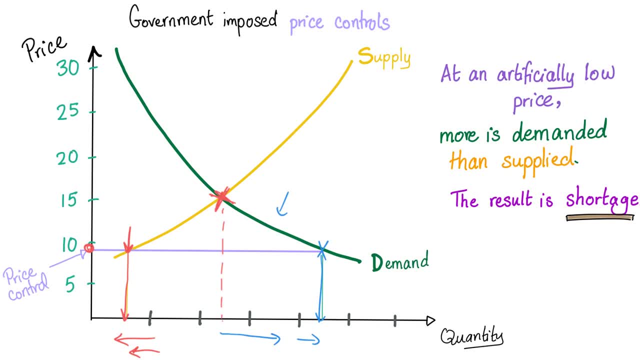 profitable anymore. But why are these greedy pharmaceutical corporations only caring about profit? Okay, let me ask you this: Let's say that you are a doctor and you work for a hospital and the hospital-like manager told you: you know, doctor, we are sorry, we cannot pay you anymore. 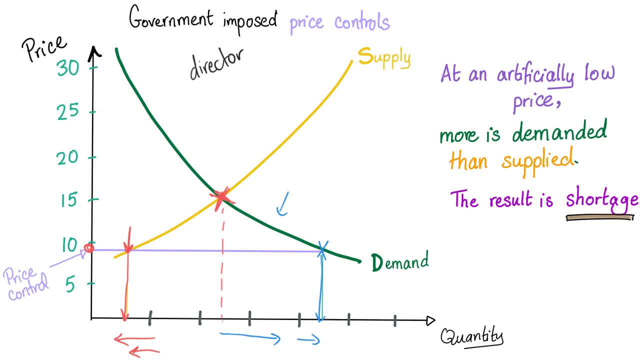 from now like forever, We don't have any money. If you want to work with us, you are more than welcome, but there is no like: do not expect any money from us from this point forward. The question is: will you go to work? 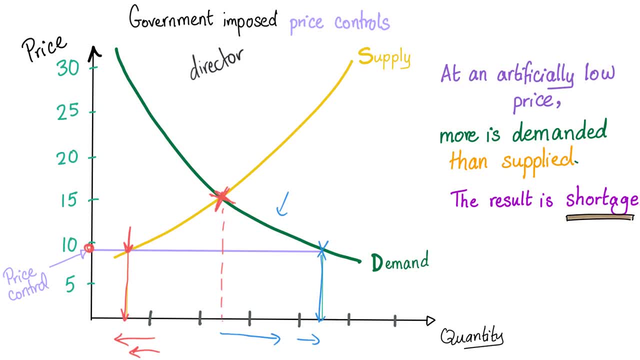 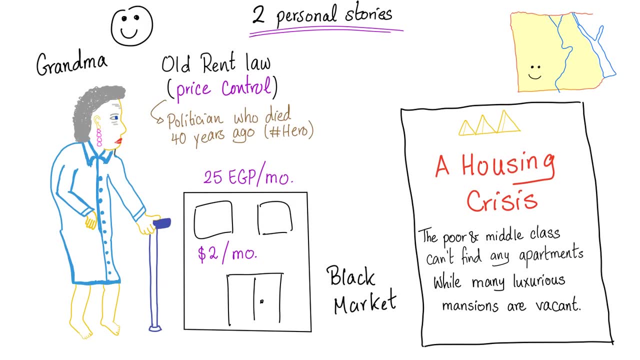 work next week? And the answer is no, Because you know what You also care about: your profit. Otherwise you will not have money to eat. Now let me tell you two personal stories about this stuff In Egypt. this is my grandma. May she rest in peace. Before she died, she was under something. 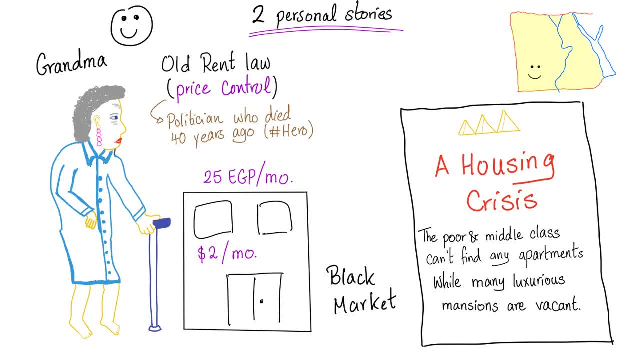 called the old rent law in Egypt. It's basically a price control and artificially low price. Basically, she paid 25 Egyptian pounds per month. Now, to put this in perspective, this is about two dollars per month. And she had some income like some pension about, I have no idea. but 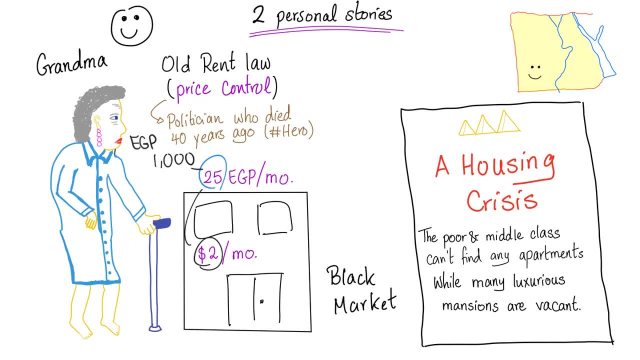 it's actually about 1,000 or higher. In other words, grandma was paying 2.5% of her income on housing. I was so happy for grandma, But I didn't see the entire picture. I read in the newspaper. 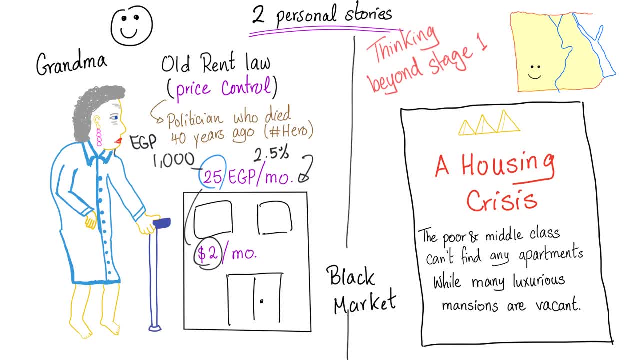 there is a housing crisis in Egypt. The poor and middle class cannot find any apartments, while many luxurious mansions are vacant. Do you know why? Because at an artificially low price, more is demanded than supplied. How about the luxurious one? The luxurious one, we're not. 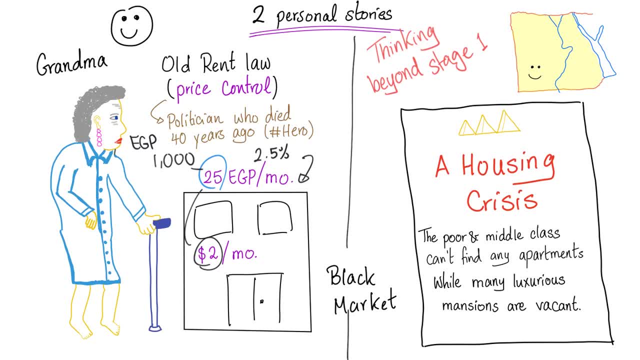 under price control Because the politicians, with good intentions, thought that we would like to help the poor and middle class, So this price control will only apply to the poor and middle class. That was was the intention. What were the consequences? The poor and the middle class. 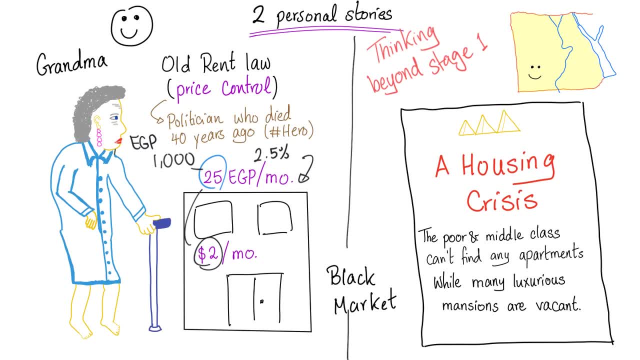 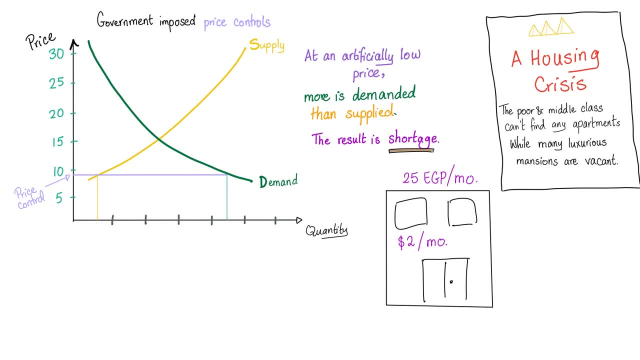 suffered while the rich didn't feel it. And whenever there is price control, there will be a shortage and there will be a black market, Because with rent control, many people would like to live for 25 Egyptian pounds per month, but very few. 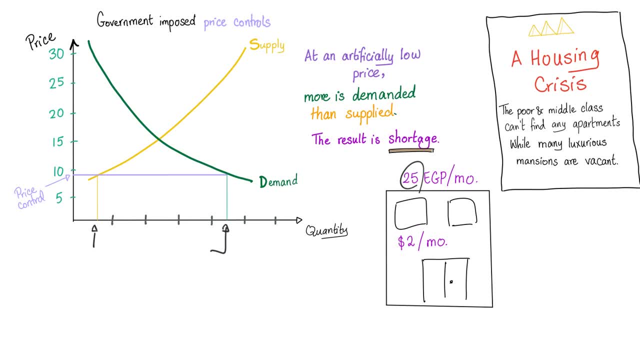 developers are willing to build new apartments because they will be losing money every second. Now do you know who made me aware of this thing? Dr Thomas Sowell, who was mentioned earlier. He's a genius. In my opinion, he is the best thinker alive today. He wrote more than 30 books. Right now, I'm in book. 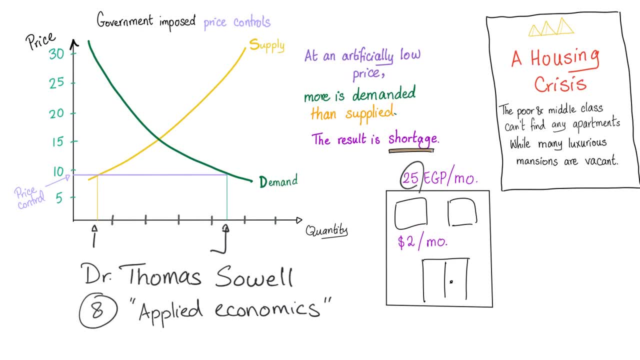 number eight. I really hope to finish all of his books. They are amazing. Do you agree with him and everything? No, I do not agree with anyone and everything. I do not agree with me on everything. The second story: When I was young, starting to learn how to drive, I was begging my dad, Please. 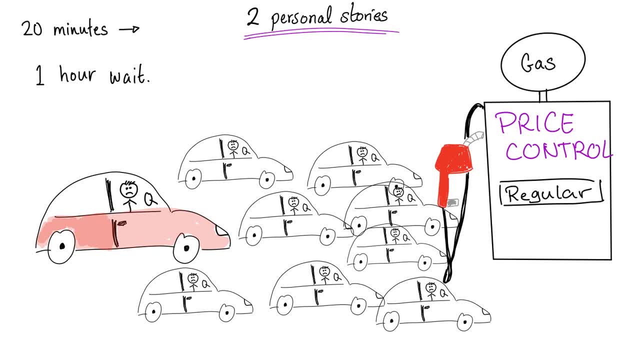 daddy, give me the car, Let me have some fun on the weekend. And finally, daddy said: yes, please be careful, But here is one condition. Okay, go ahead, daddy. Please go and fill this car with gas. I will pay for the gas, but please go and fill it up. Okay, that's easy. Nothing is. 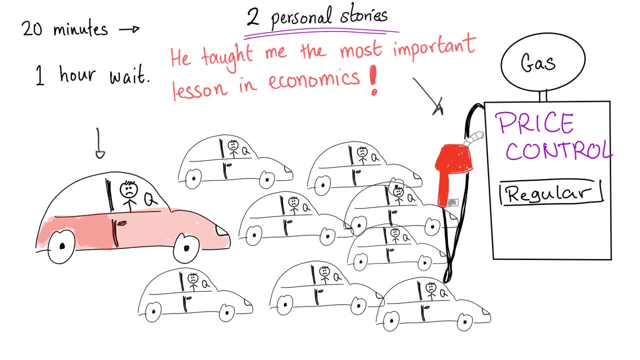 gonna happen. I will do this. You can count on me. Then I spent 20 minutes on the way to the gas pump. and then one afternoon I was in the car with my dad. I was in the car with my dad. I was in the car. 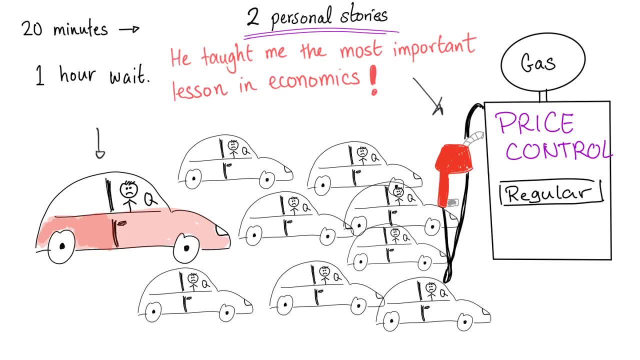 waiting in line because there was shortage, Because in Egypt there was price control for gasoline At an artificially low price, more is demanded than supply. There aren't that many gas stations because it's not profitable to build them And you'll see the shortage There is. 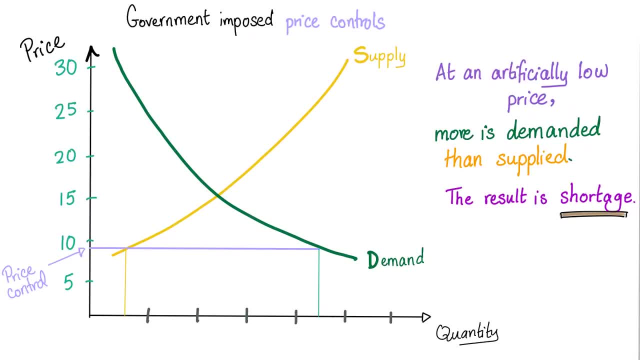 increased the quantity demanded At an artificially low price, ie price control. more is demanded than supply. The result is a shortage. In other words, shortage is a price phenomenon. You want the shortage to disappear. remove the price control, let the prices go back up to equilibrium and the suppliers will. 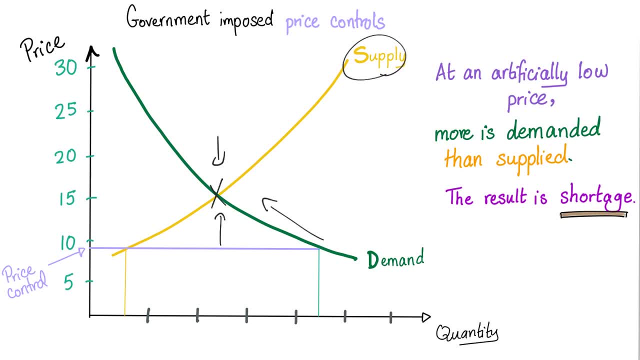 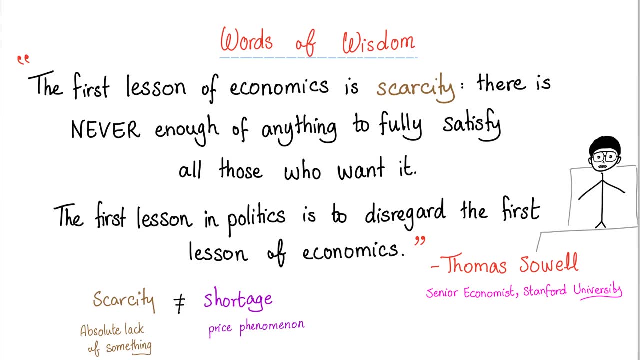 suddenly supply and the demand will suddenly decrease until you reach that sweet spot, Which brings us to some words of wisdom from my man, Dr Thomas Sowell. The first lesson of economics is scarcity. There is never enough of anything to fully satisfy all those who want it. 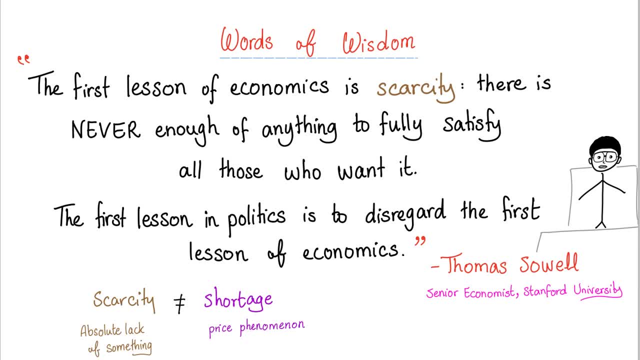 There is not enough of anything to fully satisfy all those who want it. There is not enough of iPhones for everyone who wants one. There is not enough cars for anyone. There is not enough houses. There is not enough insulin for every patient who wants them. This is the first lesson. 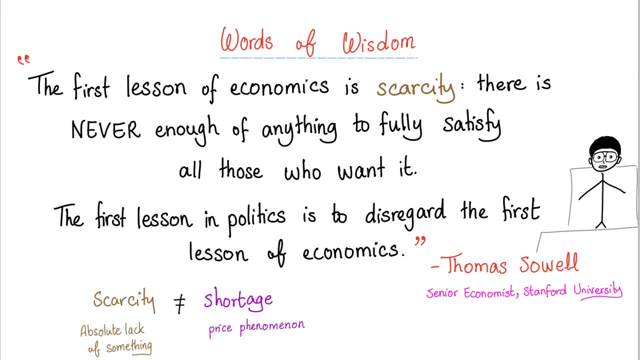 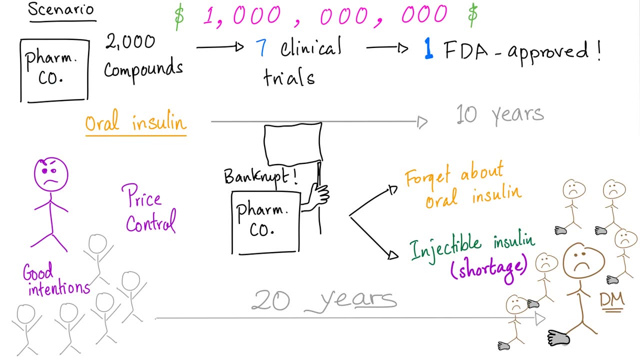 of economics, It's true, But the first lesson in politics is to disregard the first lesson of economics. Somehow, politicians think that they can just wave their magic wands and everyone will have a pony. Let me help you with this. regarding the big pharmaceutical corporation, 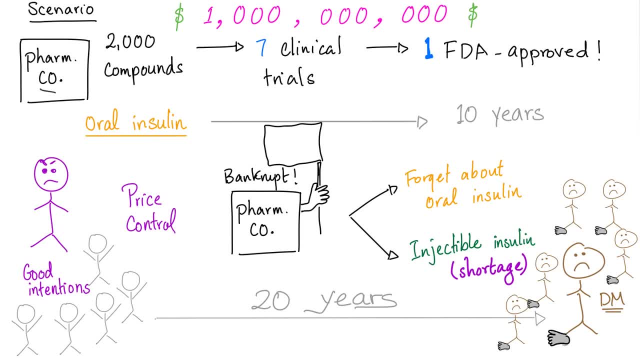 by the way, CO here stands for company, not for cardiac output or- heaven forbid- carbon monoxide. Did you know that for every 2,000 new compounds invented by a pharmaceutical corporation, only one will get FDA approved? if they were lucky, Of those, 2,007 will reach the randomized 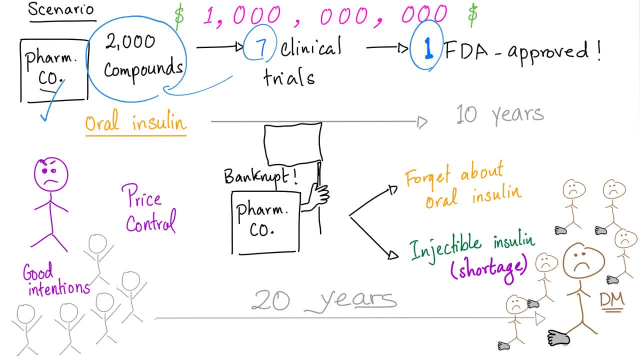 double-blinded, placebo-controlled clinical trials and, if they are lucky, approval from the FDA. From this step to this step, it can take 10 years or more. So, for instance, while we're talking right now, maybe one of those companies are working on oral. 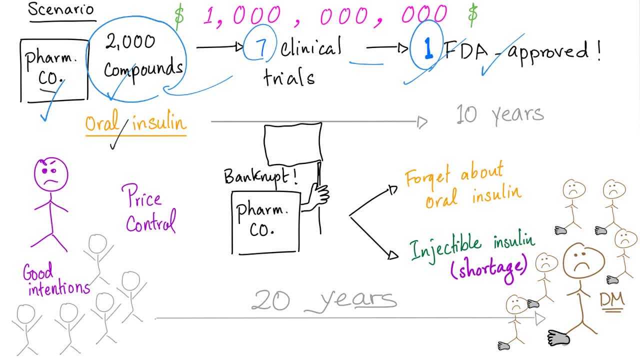 insulin instead of injections, actually oral. This will be awesome, But they cannot tell you about it now for two reasons. Number one, it's a trade secret. Number two, they cannot advertise it before it gets FDA approved. But then let's say that we have a company that is working on. 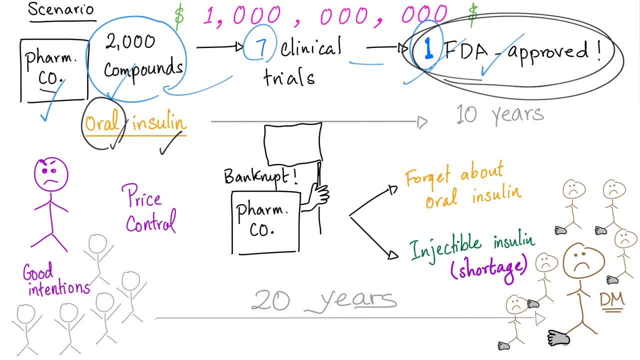 a drug and we have a politician with good intentions and he said: man, those big corporations are evil. I'm gonna pass price control laws and they cannot charge you more than 10 bucks for any medication. The people will cheer: hey, finally a guy who cares about the little man. 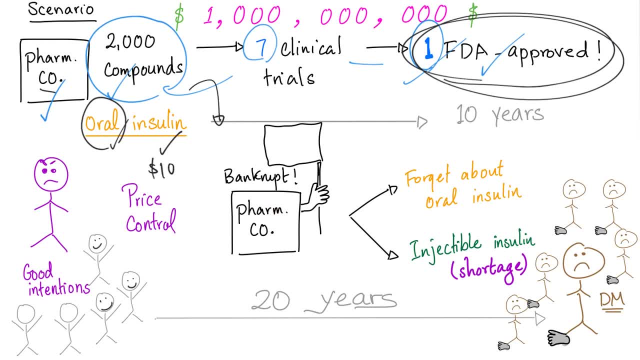 Before you know it, this big corporation will declare bankruptcy. Why? Because it cost them billions of dollars to invent those 2,000 compounds. Next, now, here are the good intentions, but look at the consequences. Now oral insulin is history. 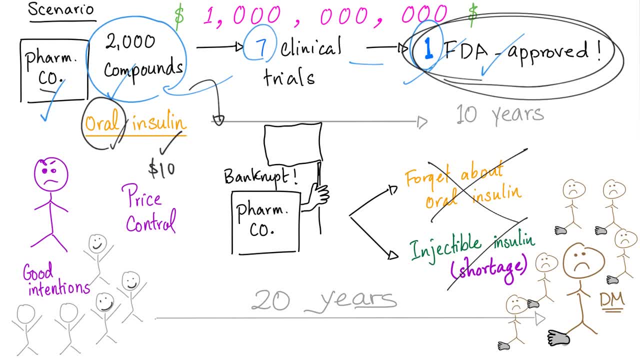 Forget about it, It's not gonna happen. Number two injectable insulin, which was available before the price control, now will have shortage. You know who's gonna suffer? Patients with diabetes, who might end up with gangrene, retinopathy and nephropathy, among others. 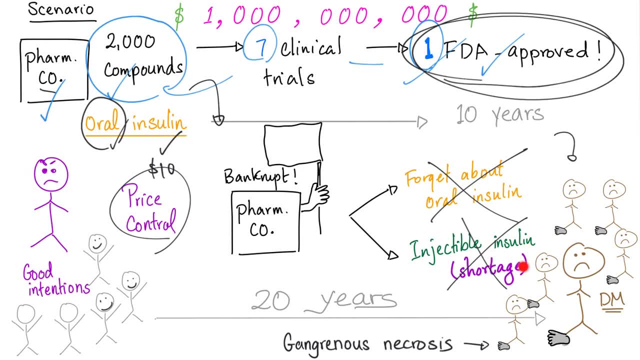 But between this politician and the shortage, it can take about 20 years. No one will actually remember that this tragedy happened because of this politician, who is now happy retired in his mansion and everyone thinks he was a hero. So if you really care about flesh and blood, human beings- 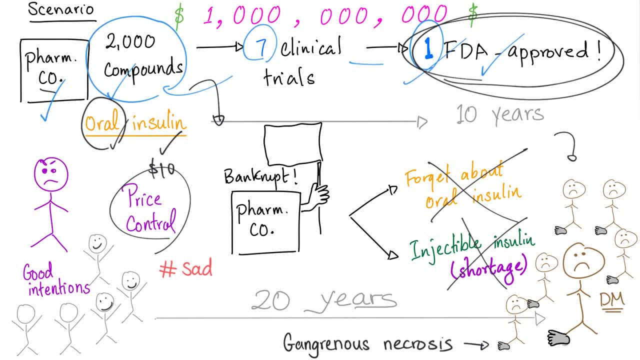 you should care about pharmaceutical corporations, big or small. If they do something illegal or immoral, of course we should punish them. But until you prove this you can't say you're not a hero, and you can't even be a hero yourself. 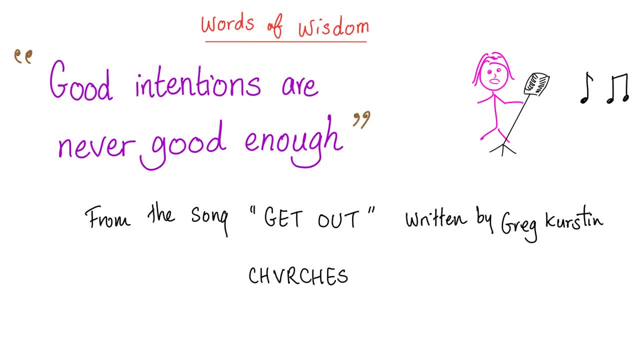 So I would like to request a statement from my student, Salman Zinani, that just let them function, because they are helping millions of people around the world. And don't take my word for it and forget economics to the hell with it. learn from this song. 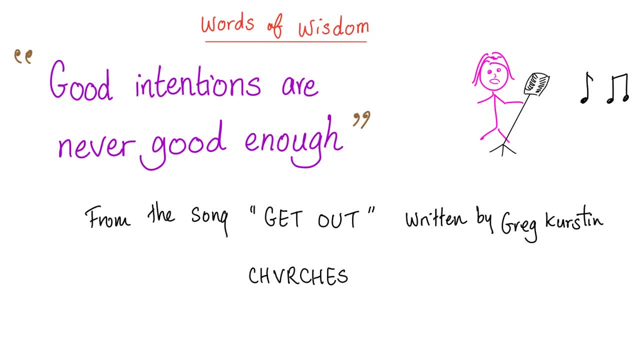 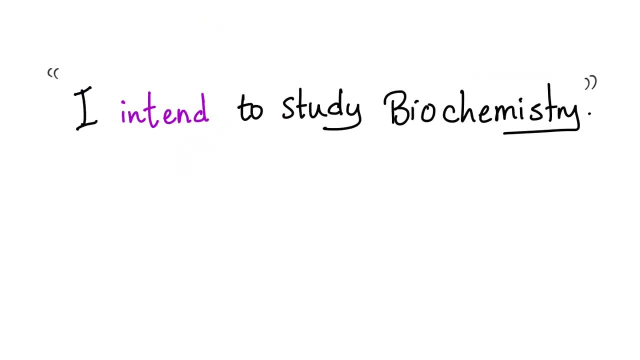 Good intention's never good enough. so get out. Get out and study biochemistry and try to make the world a better place. Maybe then there is hope for future generations. study biochemistry, it doesn't mean anything. I'm not impressed. Let's switch roles. Let's imagine: 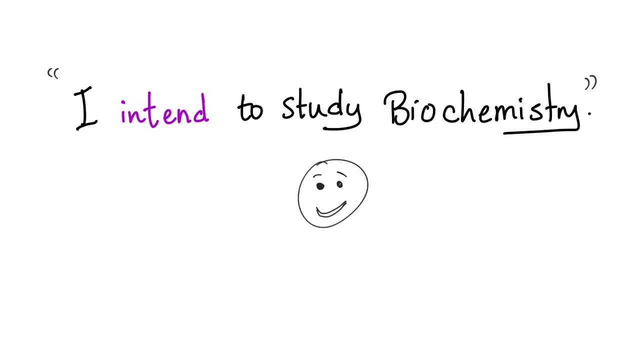 that you have acute appendicitis with fever, leukocytosis right lower quadrant pain with guarding rigidity, etc. and some clinical signs. And then you went to a surgeon with very good intentions But for some mistake, instead of removing your appendix, he removed your entire. 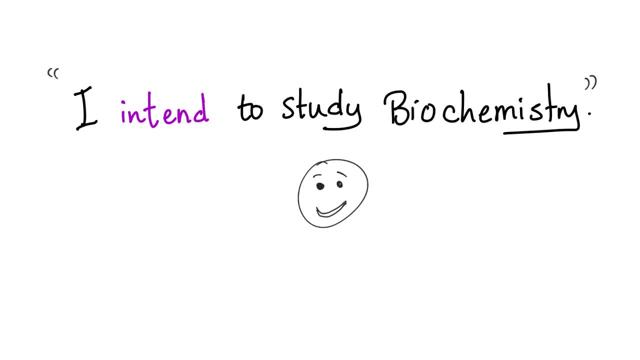 colon And after the surgery he said: you know what? I'm sorry, I made a mistake, But I had good intentions. Now, what are your options? What will you respond? Okay, doctor, don't worry about it. 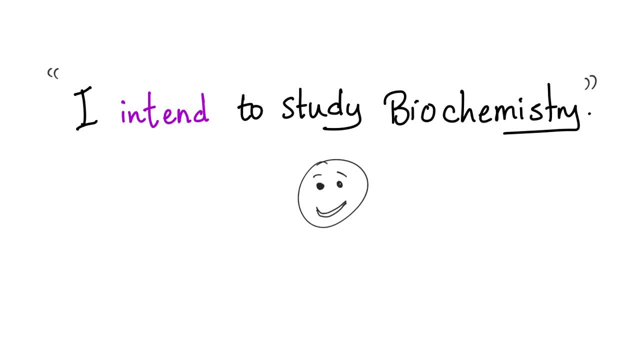 As long as you had good intentions, it's okay. Or number two: I want this scumburger in jail so that he doesn't repeat that with other patients. I think you will think the latter Good intentions are never good enough. So welcome to the journey of biochemistry, You will.